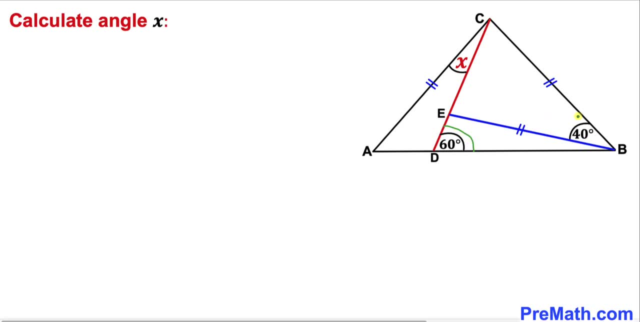 and this angle EBC is 40 degrees, and now we are going to calculate this angle X. Please don't forget to give a thumbs up and subscribe. Let me make it very clear that this triangle is not 100% true to the scale. Let's go ahead and get started. Here is our very first step. Let's focus on this triangle EBC, and we know that this is an isosceles triangle, since this side length is equal to this side length. Therefore, this angle has got to be equal to this angle and we know this is a 40 degrees angle. 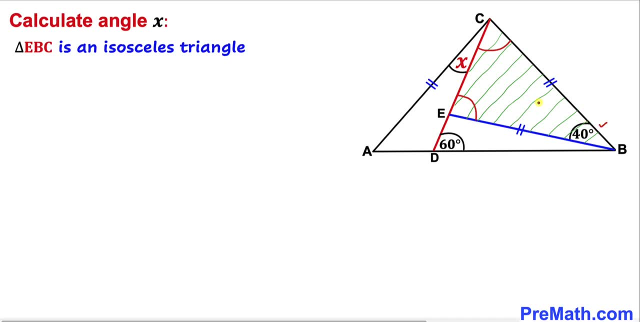 And we know that the sum of the angles in a triangle must be 180 degrees. so therefore, this angle has got to be 70 degrees and this angle is 70 degrees as well, such that if we add all these three angles, we add up to 180 degrees. Therefore, our angles BEC and BCE are equal to this angle. 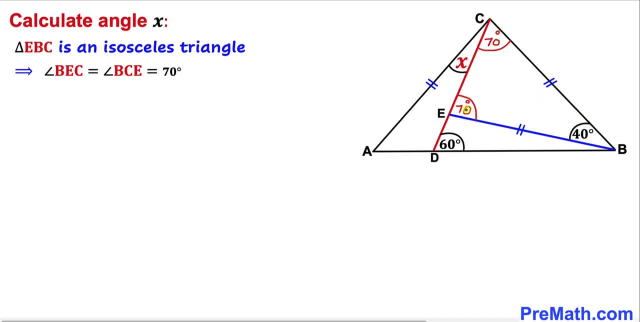 Now let's recall this straight angle property. For example, if I take a degree, We can calculate that from here I can get 180 degree angle and from this degree 80 degree angle. Here I have set a velocity of 180 degree, so the angle BED has got to be 110 degrees. 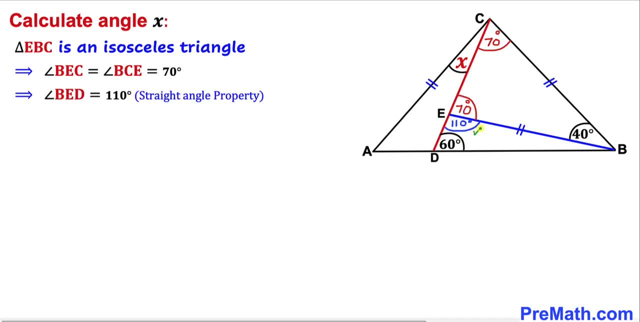 Then the angle CE X, Ambх, CE 7 degree, and who knows? then we will have demonstrations 110 degrees. And here's our next step. Let's focus on this triangle BED. And now let's recall triangle sum theorem. According to this theorem, the sum of three interior angles in a triangle 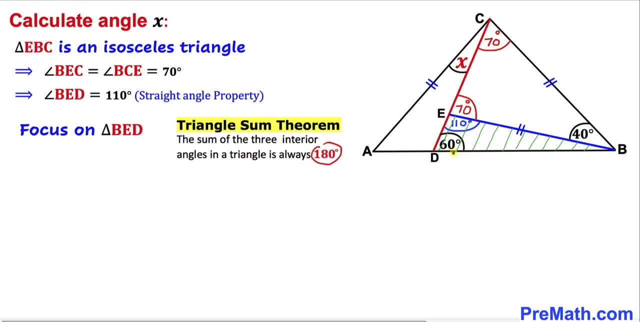 must be 180 degrees. If this angle is 60 degrees, this angle is 110 degrees, So therefore, this angle has got to be 10 degrees. Therefore, our this angle, EBD, turns out to be 10 degrees. Therefore, this whole angle is going to be the sum of these two individual angles: 10 plus.